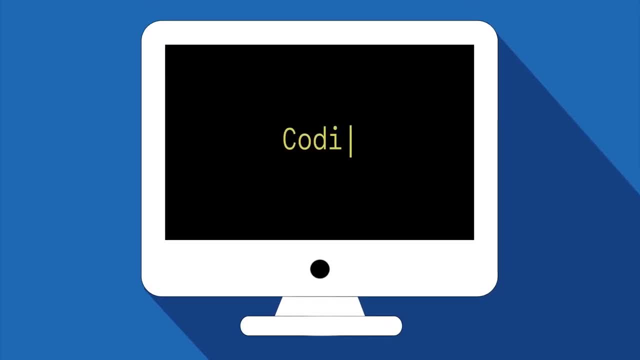 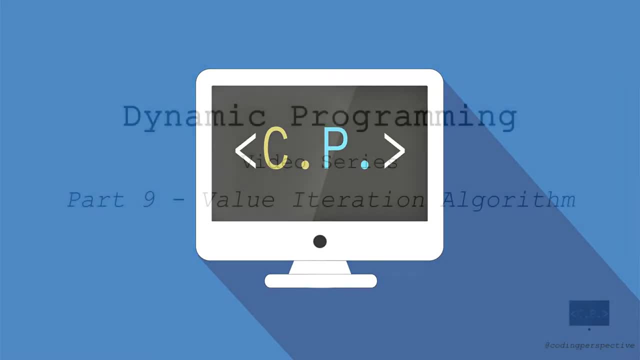 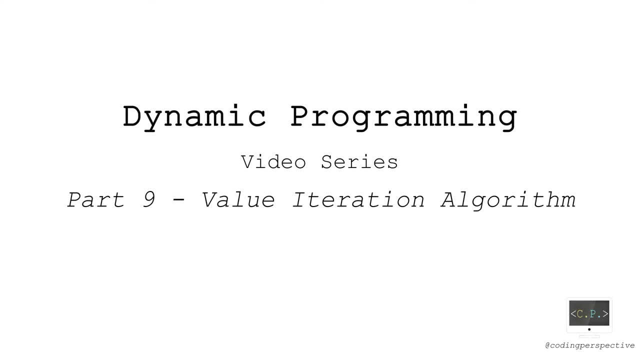 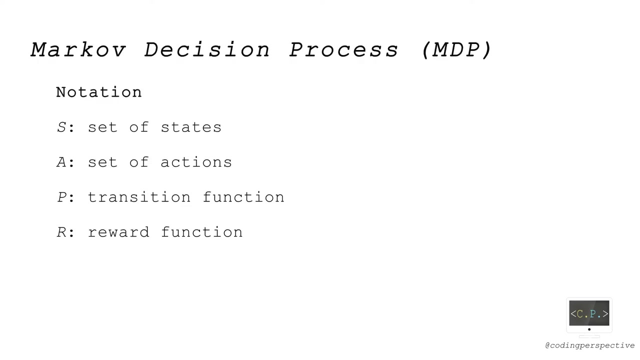 Hello everyone, this is the ninth video of Dynamic Chromic Algorithms video series. In this video I will shortly introduce Markov Decision Process and how to find the optimal solution by using the Value Iteration Algorithm. An MDP can be defined by a set of states S set of actions: A. a transition function, P. 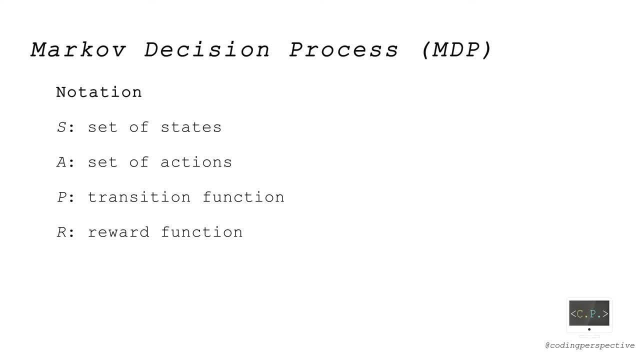 and lastly a reward, function R. In this process, at n, iteration k, we are in state sk, an element of set S. Then we take an action ak in set A and perform it. Taking this action ak yields our sk ak reward and we move to another state- sk plus 1 depending on our action. This transaction, 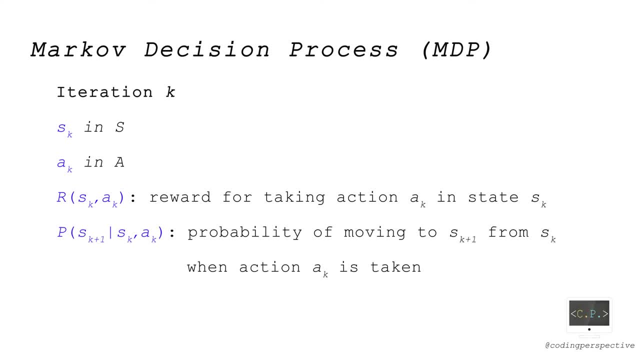 happens with some probability, P given sk and ak. Our aim in this problem is to find the optimal set of actions that maximize total revenue for a given initial state. To solve this problem, we will use Value Iteration Algorithm First. let Q be the expected. 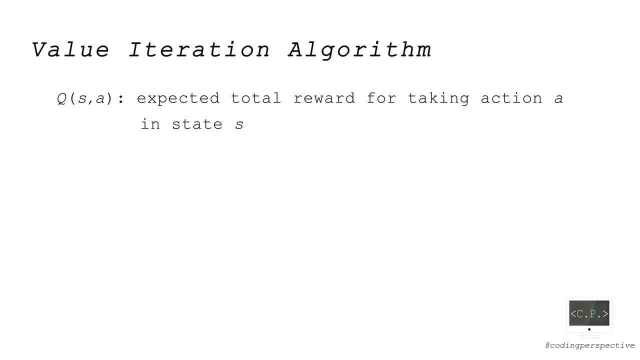 total reward for taking action A in state S. Also, let V be the maximum expected total reward starting from state S. V is sometimes called a value function. in S We can calculate Q as you see. R is the immediate reward after taking action A And the summation is the expected future reward. 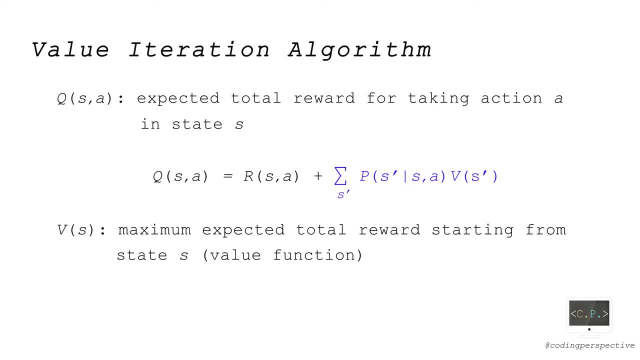 after moving to the next state. S' Q is simply equal to the summation of these two, Then maximum value of Q over A gives us V. In the Value Iteration Algorithm we will calculate the value functions iteratively until they converge. 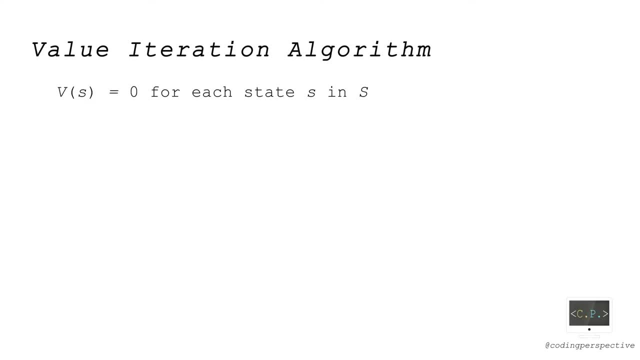 As an initial step we set the value functions to 0. Then we repeat calculating V for each state S until it converges To calculate V. we first calculate Q as an intermediate step A for action A, then take its maximum over A. Now let's code this algorithm in. 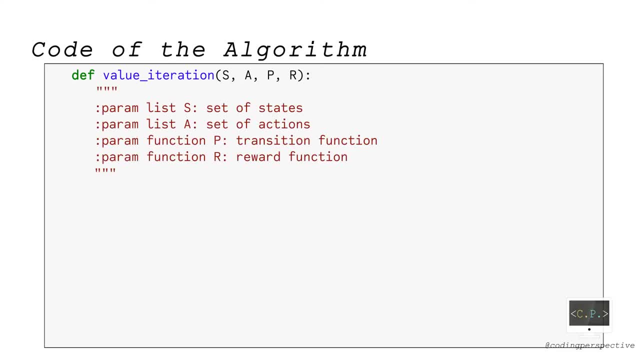 Python by writing a function called value iteration. The input of this function is the set of states- S as a list, the set of actions- A as a list, the transition function, P as a function and, lastly, reward function as a function. I will later talk about how to. 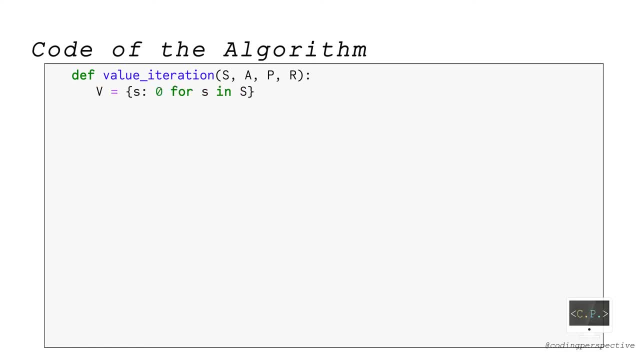 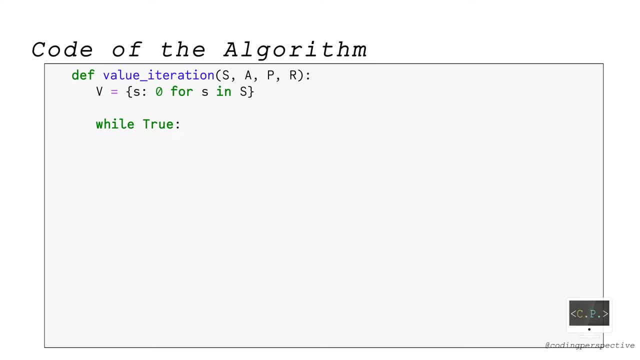 We will terminate this loop by using break once we get the convergence. Since we will update the value functions at each iteration, I define a variable called oddV to store the value functions at the previous iteration. We can initialize it as a copy of variable V. As a termination condition, we check whether the value function remains. 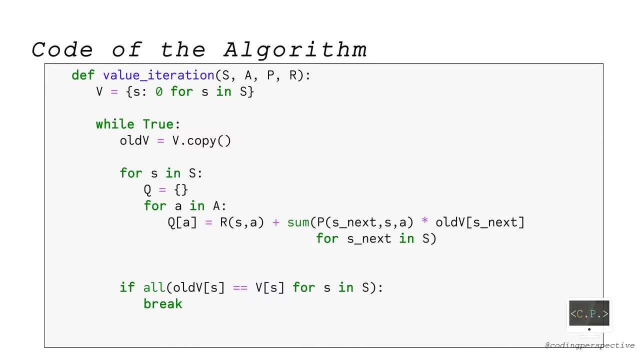 the same by comparing oddV with V To update the value function V for a temporary state S at any iteration. we first calculate Q for each action A. as you see, One important point here is that we use old V instead of V while computing the expected. 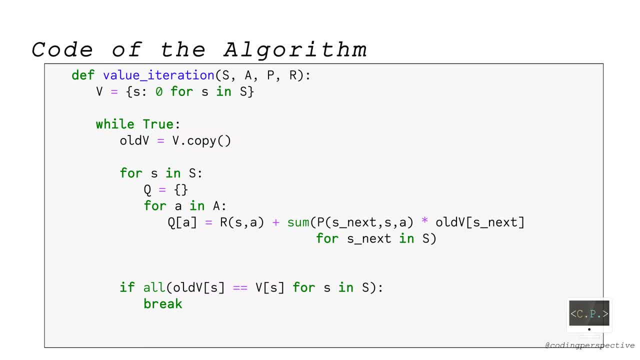 future reward in this sum because we update V while iterating state S. Then we can calculate and update V by finding the maximum value of Q over A. Once we attain the convergence, we return the value of functions as an output. Before showing how to define these inputs, it is worth mentioning that this is not the 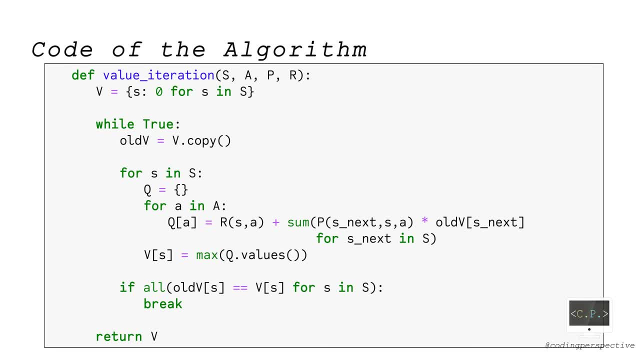 best way to code this algorithm in terms of the real-time computation performance. Right now I am not concerned about it because we will share a video about how to make these functions faster Here. I believe it is important to understand the implementation of such an algorithm. 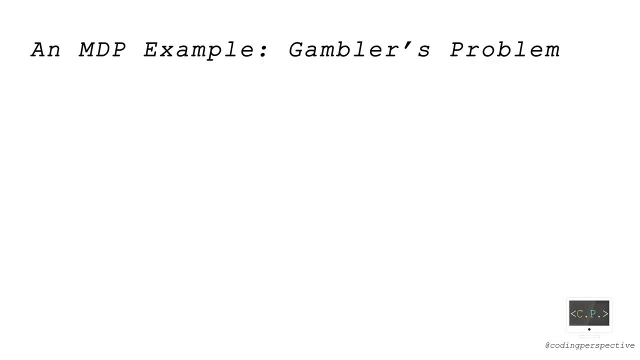 Improving is the next step. To use these functions, we need to understand the implementation of such an algorithm. To use these functions, we need to understand the implementation of such an algorithm. For example, let's consider a gambler's problem. 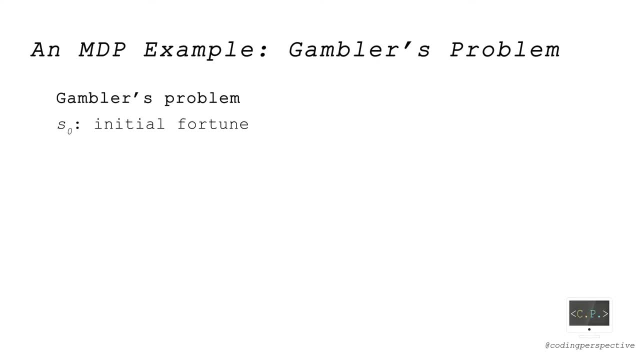 In this problem, the gambler starts with an initial fortune of size S- zero and plays until the fortune reaches value n or zero. At each gamble, the gambler either wins the bet with probability P or loses it with probability 1-P. The gambler gains some reward only if the fortune reaches the value n. 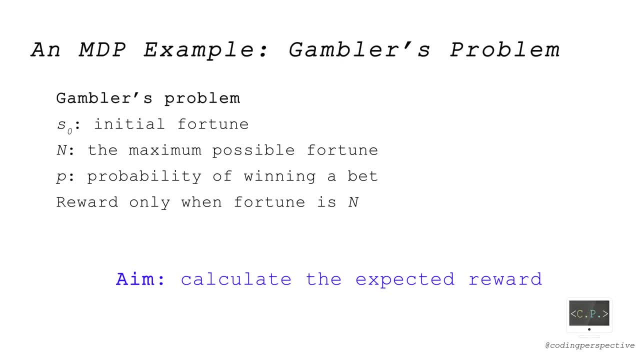 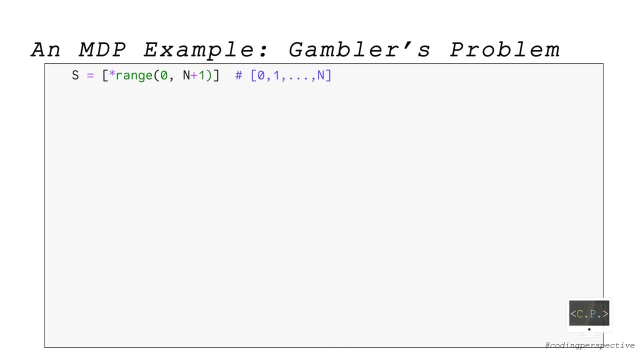 Our aim in this problem is to calculate the expected reward for any given S zero. The state of the system is like: this is the current fortune. So the set S is from 0 to N, where 0 and N are the absorbing states. 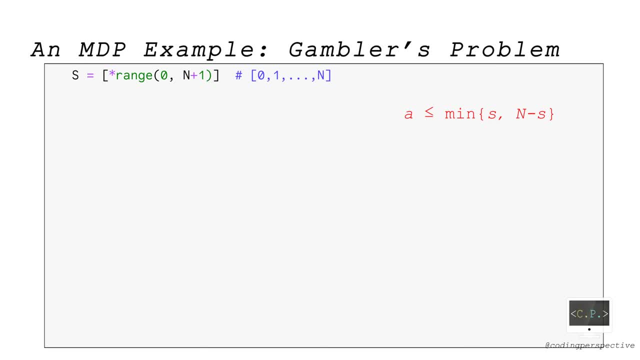 The maximum possible amount of bet is the minimum of S and N-S, since the fortune cannot be less than 0 or more than N. So the set A depends on the current state S, and it consists of values from 0 to minimum of S and N-S. In this implementation, instead of restricting 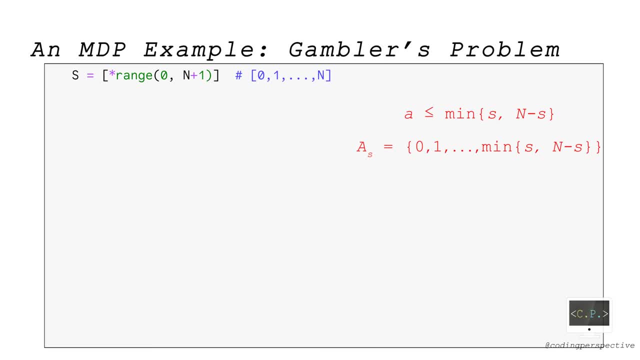 the set A. I will define the transition function P in a way that any non-feasible transition will not be allowed. So we define set A from 0 to N and transition function P as you see It returns P in case of winning, 1-P in case of losing and 0 otherwise. 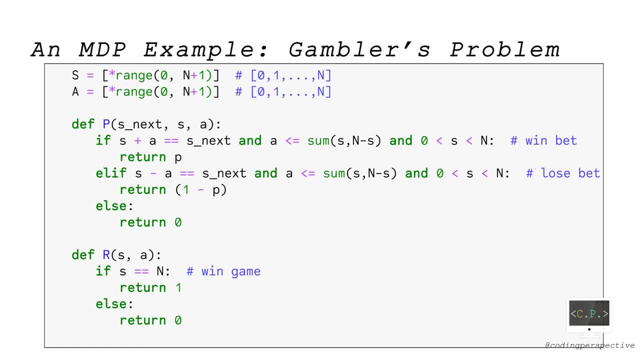 Lastly, we define function R in a way that it returns 1 if S is equal to N, because it's the only state that the gambler wins the game. Now we are ready to run our function with these inputs. These inputs are totally problem-specific, So, depending on your problem, 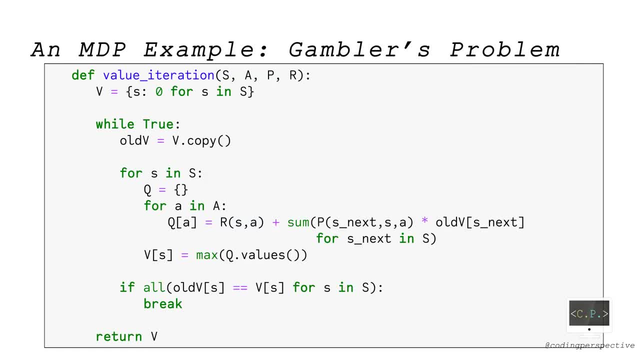 you may need to modify them. Before showing the outputs, I will modify the value iteration function so that we can obtain the optimal policy along with the value functions. We initialize a dictionary called optimal policy, where the keys are the states. Then we update this dictionary whenever we update the value function by finding the action that maximizes. 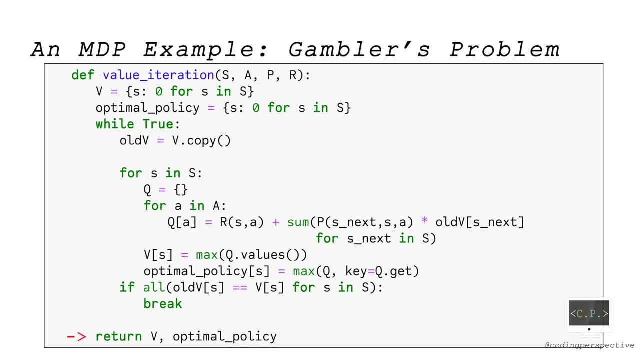 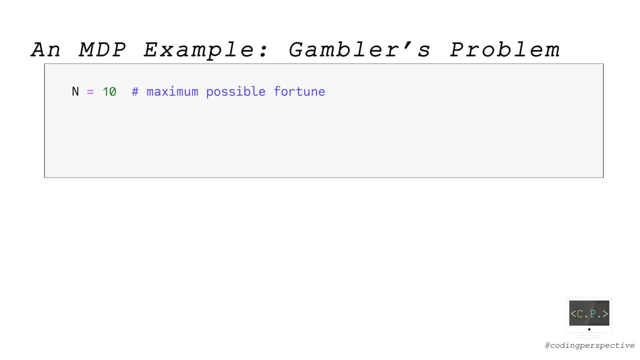 Q And we return P And we return optimal policy as an output For the gambler's ruined example. let the maximum possible fortune N be equal to 10, and probability P be equal to 0.4.. When we run our value iteration function for this, 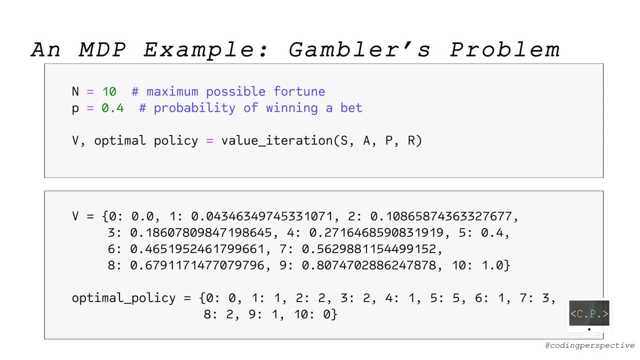 problem. the outputs look like as you see. You can see how much the gambler needs to bet in each state by looking at the optimal policy dictionary. For example, the gambler needs to bet 5 when the current fortune is 5, and 3 when the current fortune is 5..